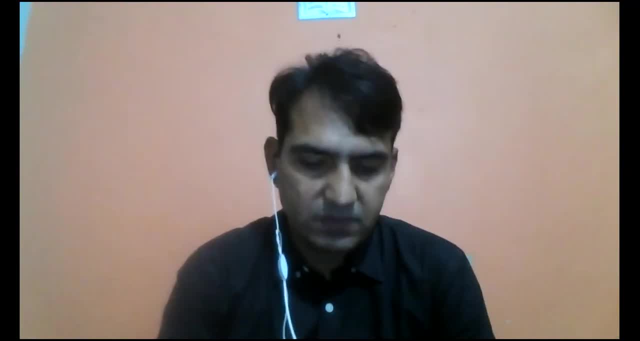 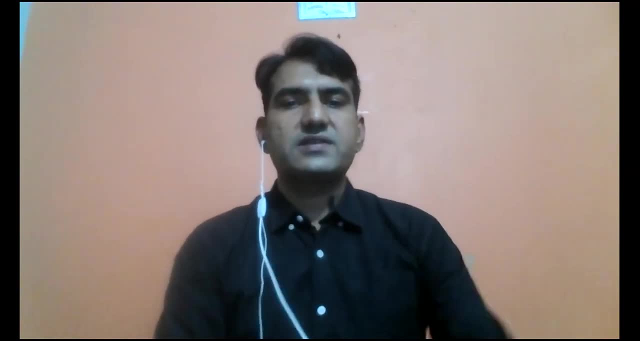 climatology and hydrogeography. What I said to some extent to the climatology, because the steps which we are going to discuss in the in this lecture of hydro hydrological cycle, on the cycle which I will be talking about in the next lecture. So let's get started. 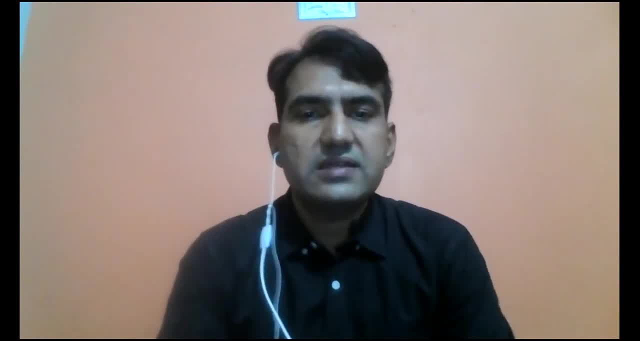 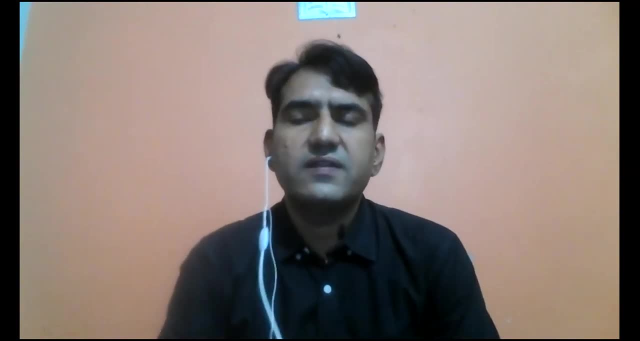 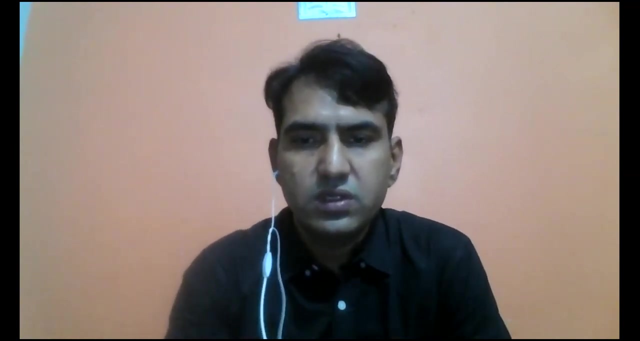 The main steps. these are steps are being taught in the climatologic like, such as like evaporation, condensation and the precipitation and off. So these are the part of the climate of logic. So let's go to the lecture, which is all about the 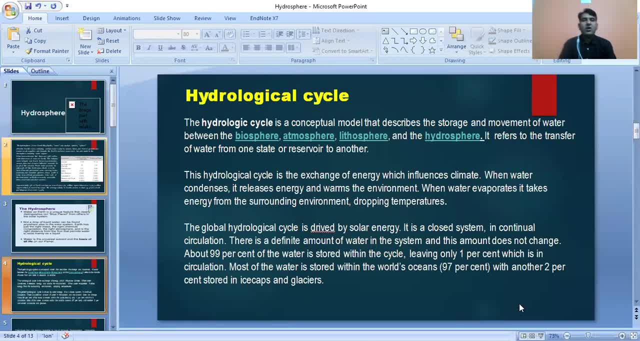 hydrological cycle. So hydrological cycle, or the water cycle, is very important for the geographer also been, I'll say it is a very common topic which I must everyone, everyone should have a knowledge about this one, because through this hydrological cycle, the water, water which is being moving or rolling, the 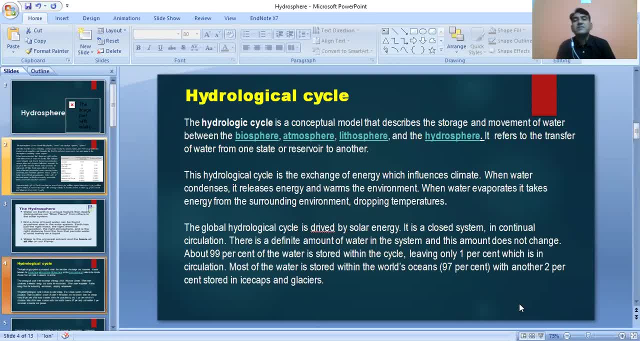 mostly the water is being received or being got by the different parts of the landmass area. so hydrological cycle or the water cycle is the main source as a main source of fresh water or, you can, source of water on in the world, though the different the distribution and the distribution of supplies. another thing: 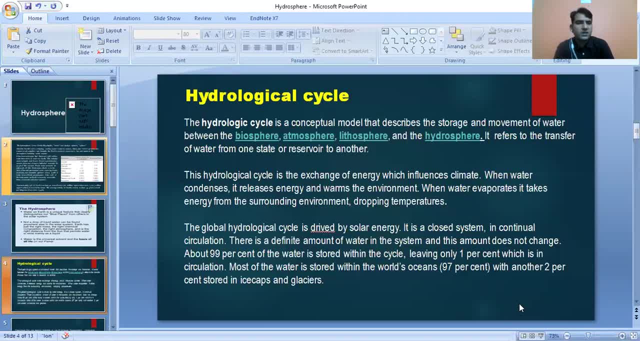 or anything. but how do you cycle? mostly provide the water to the world or to the landmass area. so let's start with the definition arts introduction. so hydrological cycle is a conceptual model that described the storage movement of the water between biosphere, atmosphere, lithosphere and the 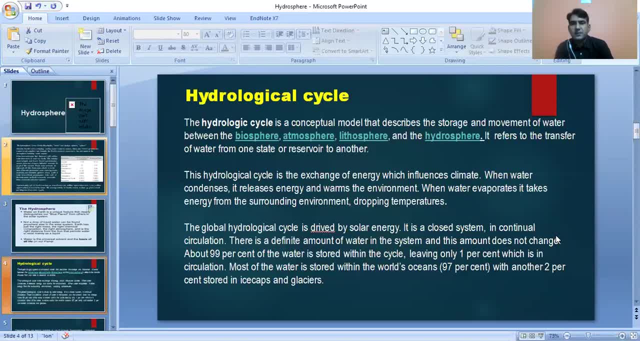 hydrosphere. so, as in a previous lecture we discussed these, all these spheres, we also discuss biosphere, atmosphere, so lithosphere, hydrosphere and geographic domains, so the water side, the water which is being rolling. are we moving between these spheres such as biosphere, atmosphere, lithosphere, and it referred? 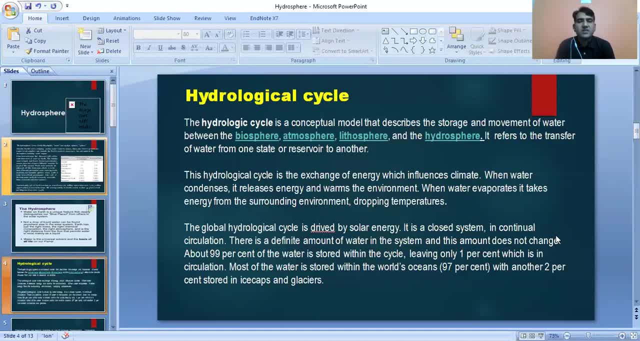 to the transfer of water from one state or reservoir to another. so when the water is moving are being rolling into these, between these, these spheres, it it changes states, it changes its place or the region. so it's all about the moving of water, with its change in its state, in the form and also. 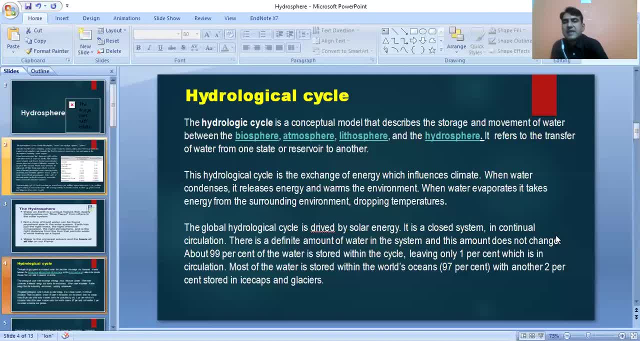 changing the place where it's being found there. so hydrological cycle is a conceptual model. let's go further. let me clear, as you'll find a very, very important, a very interesting fix in becoming slouch: the. the hydrogen cycle is the exchange of energy with influence climate. this is also very important. 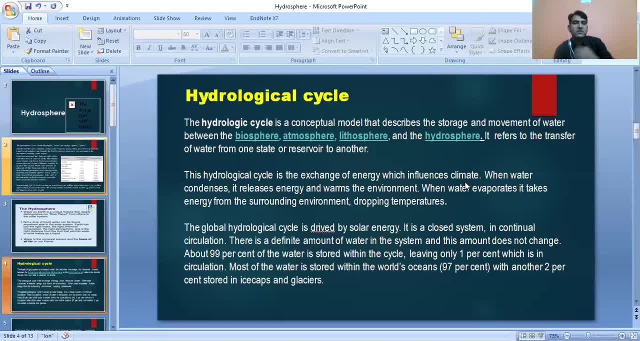 statement what it says not only hydrogen cycle, where the water has been moved from bottom to the top and top to the bottom, but it's also been achieved by the exchange of the energy which influence our climate. so let's see how it is being. it is the energy which has been exchanged and how it influenced the 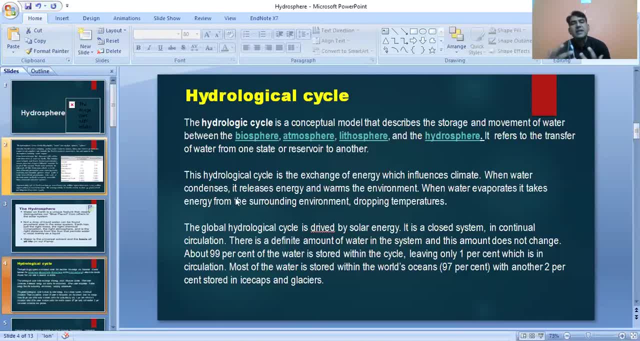 climate. so when water condense, it release energy and warms the environment. so when you see the steps of hydrological cycle, we have a evaporation and water evaporates. I'll go individually. these are the steps in coming slides. so when water is in, evaporate and be when it's evaporating. 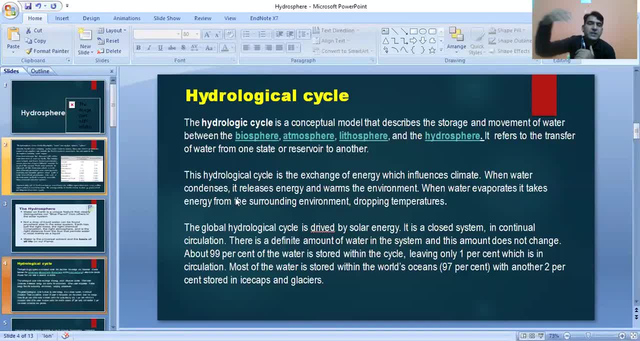 it's reached the second stage of the condensation: when it be condensed, after condensation, when it, when it precipitated, so so, when it be condensed, what is way it release the energy which warm the environment? so, when the water vapors goes up, and when they close together, when they close together in the 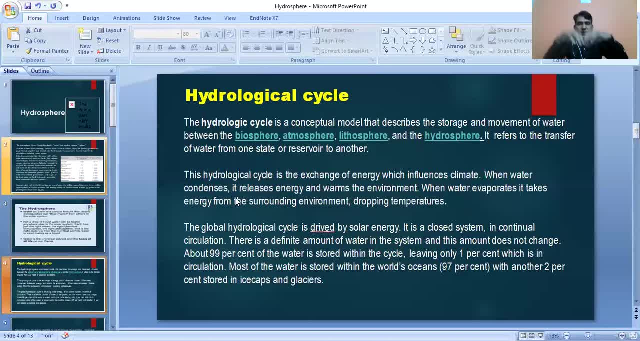 form of droplets. they and when they start to burst, they release the energy and that energy become the part of environments. when water ever operates, when water evaporate, it takes the energy from surrounding environment, dropping the temperature. so when the water has been at the, at the surface, at 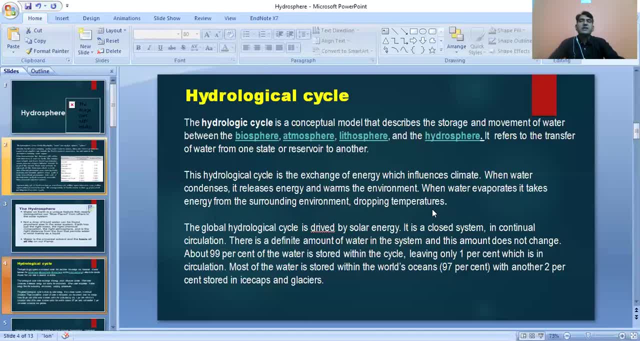 the bottom, when it can work into the vapor, and then vapor is start to move upward. they what I said, they what I say. it takes energy from surrounding us, so they takes the energy from surrounding area and when they goes upward they drop the temperature of that area or the surrounding area. 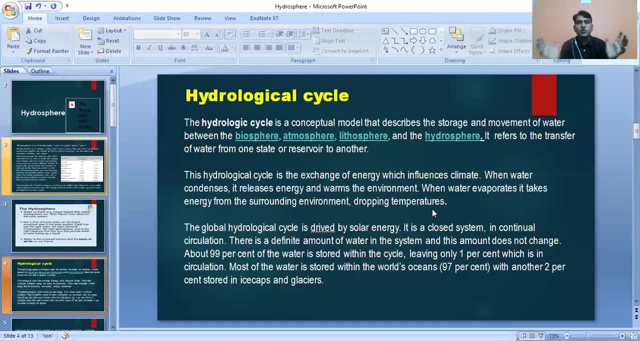 area. so not only the water has been moved, it also the energy being extinct. either the energy is being released, so they either it make the environment warm or it's also dropping, decrease the temperature and also make it more cooler. so the global hydrological cycle is drived by solar energy. you all know this. 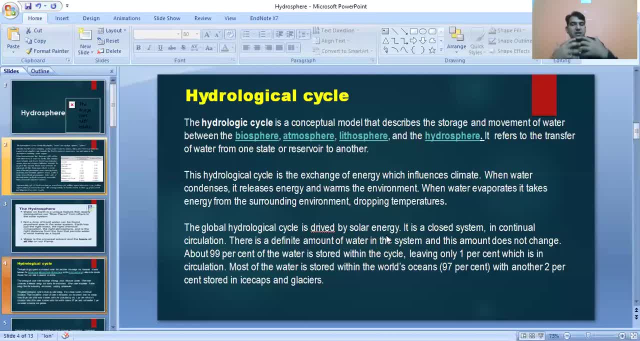 side of the cycle is being run by, or the driver, or the controller determined by the solar energy. so when the sunlight is being falling on the surface of earth, so the water which is available there, the water has been present, they start to evaporate. so I will go further. in the coming slides I will have a detailed 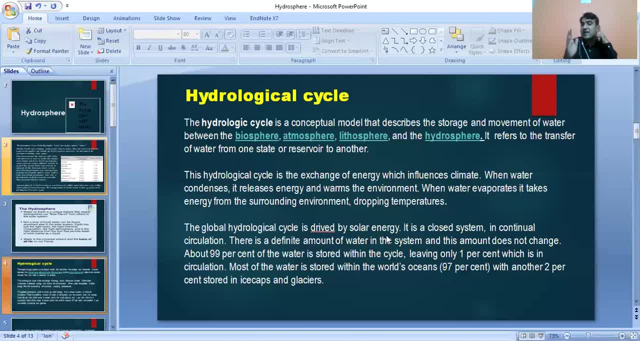 discussion on that. but what has been said? that sunlight is that driving force. it's a driving force behind the running of the hydrological cycle. so what is it? it is a closed system in continual circulation. so this hydrological cycle is a closed system. it's been, has been fixed or been running with the same same intensity. I'll say: 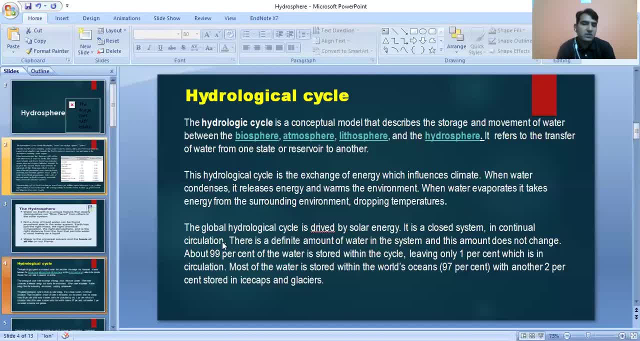 same system and it's a continual circulation. it's in a continual process. so it is closed and it is running and it is also continuous. it is a closed system, as you can see. it has a conceptual diagram or a conceptual system. after that. it is a continual process, a continual circulation. it's been. 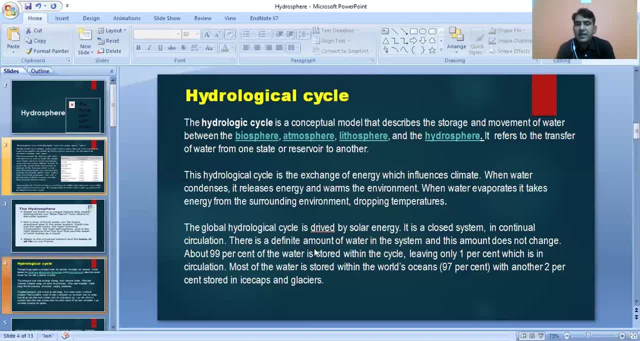 continuous been happening. so there is a definite amount of water, of water in the system and this amount doesn't change. so what has been said, the amount of water, the water which is present here, it is a definite, it's a fixed one. so there's a no change in the amount of water, but because matter isn't moving, 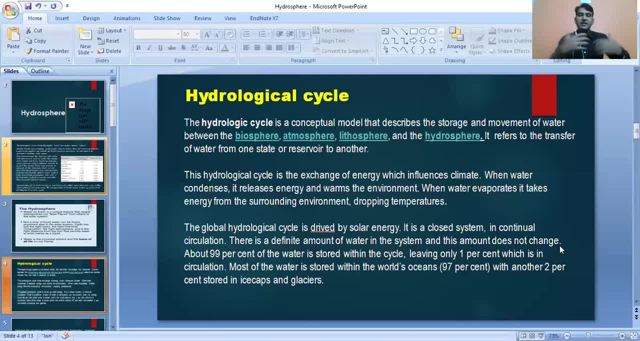 so we feel, we might be feel that the water is being decreased or increased, but in hydrolysis cycle water doesn't increase or decrease. the amount is fixed because it's been rolling, is moving, is circulating, so this amount doesn't change. so what is then? it doesn't change. 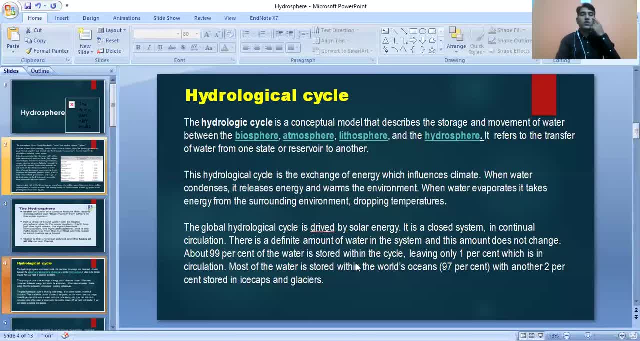 about 99% of water is stored within the within this cycle, and leaving only 1% which is in the circulation. so 99% of waters again is stored. only 1% of water has been circulating, Jojo, 99%. right, it's been same, it's been fixed. 8% Pani Jovo circulate. can't I either be there or there? so 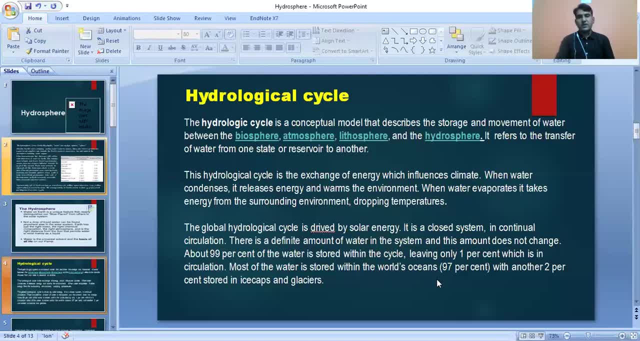 most of water is stored within the world oceans. everybody knows about that. we already discussed that 97% water has been found in the ocean, in the seas, and with another 2%, stolen ice caves in the glacier. so if you, if you watch my previous lectures, I had a discuss about the amount of water. 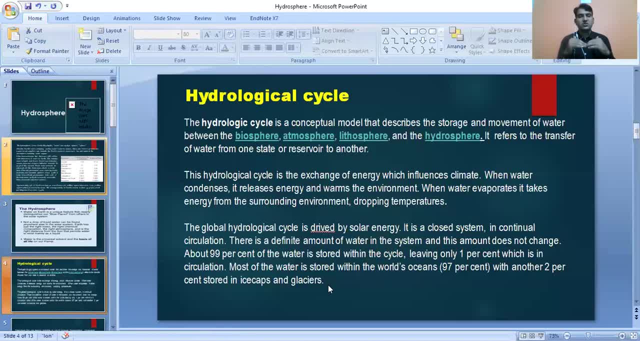 distribution of water. fresh water, break breakish or saltish water? how much water is present? so we had a very strange calculation or statistic. still was there, 97% water was present. oceans, that is the bracket saltish water. the rest of water is the fresh water or an out of if you, if you make it hundreds now, 97 in ocean, 2% is in the ice. 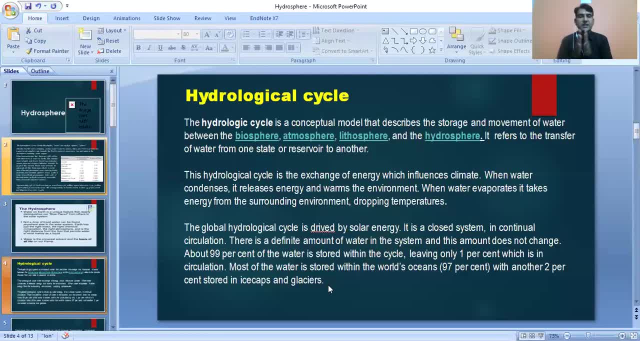 cabin Galicia. so you can imagine the ice, ice capes, a glacier. they always been in a solid form. they are freeze when salt and unless we have a certain conditions where they start to melt, otherwise they are, they will be there in their form. they will not be melted. so go further so. 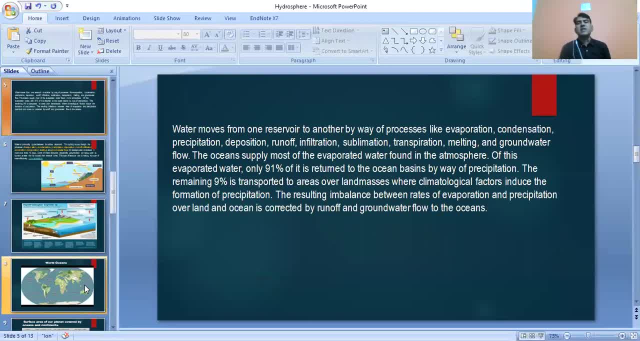 water moves from one reservoir to another by the way of process like evaporation, condensation, precipitation, uh uh, precipitation, runoff, infiltration, sublimation, transpiration, melting and etc. so these are the different it's days by which water has been growing. one is the evaporation, then 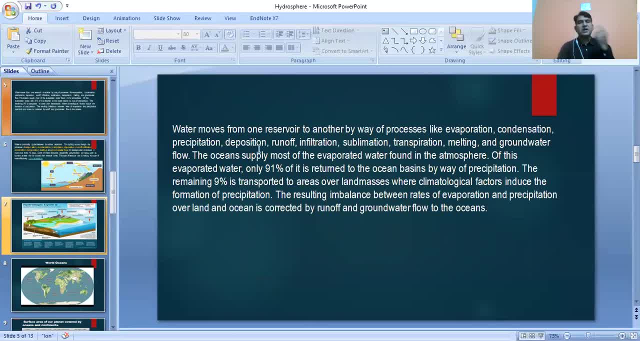 we have a condensation: precipitation, deposition, runoff, infiltration, sublimation. sublimation is a process by which uh water- because I will discuss these- uh these evaporationmed, whilst accidents AppThri. sublimation is across interpretation means when water goes down, our perk allowed. 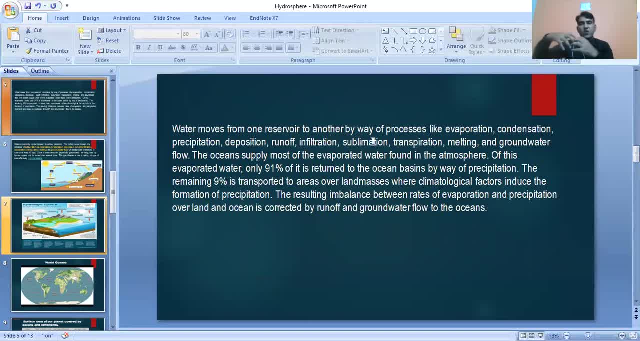 inside the earth. and sublimation is when water, uh temperature changes, Floating all the time, all of water, when the ice directly convert into the vapor. So especially when the ice which is found at the top of the mountains, on the glacier, ice capillary, they directly convert into. 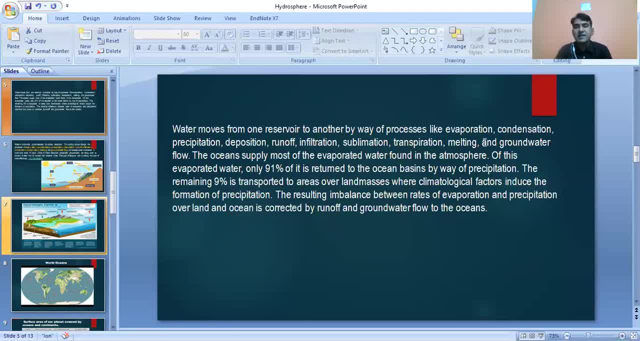 the vapor and goes into the environment: Transpiration, melting and groundwater. The ocean supply. most of the evaporated water found in the atmosphere. This is true. Most of the water comes which has been evaporated comes from the ocean, which goes to the atmosphere. So 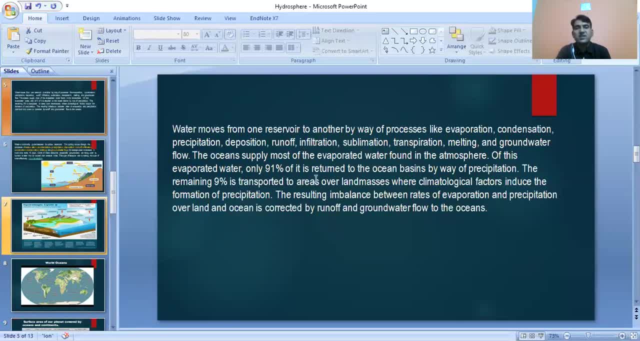 of this evaporated water, only 91% of it is returned to the ocean basin by the way of the precipitation. So what is being said if 100% of the evaporation is happening on the oceans? 91% of the water which 100%- which goes in the form of evaporation in the atmosphere? 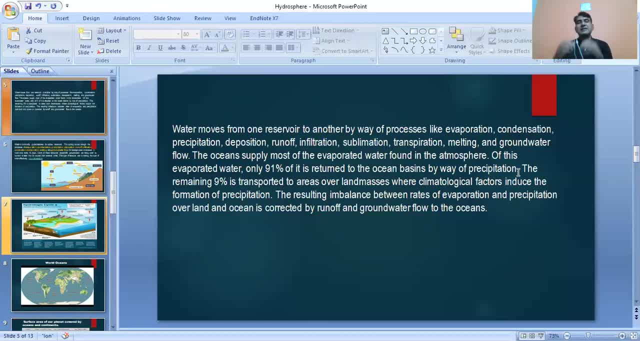 91% returned to the ocean, But it is back directly to the oceans or the seas. So 91ięcy 91% comes back. So what happens about nine percent? The remaining 9% is transported to areas or landmines where. 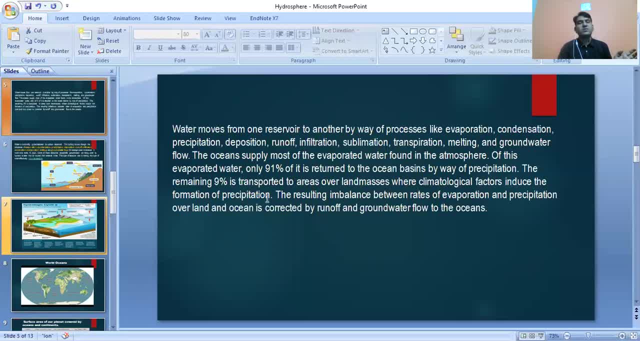 climat usage 효 when the effect that induce the formation of formation of precipitation. So the precipitation which has been happening in the landmass area, 9% of water, goes there Again, the resulting imbalance between rates of evaporation and precipitation over land. 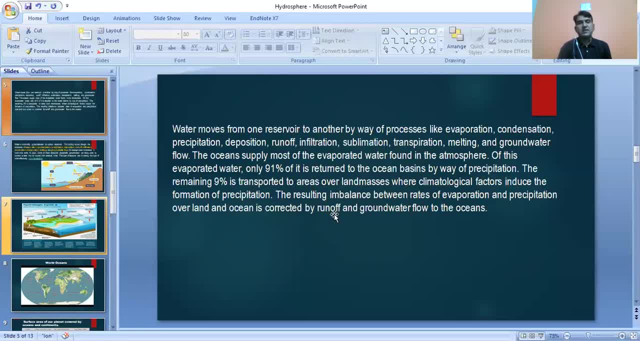 and ocean correlated by corrected by the runoff and groundwater flow to the oceans. so the same: the 90% of water which went to the landmass areas. again, what happens when water precipitation happens, when rainfall happens, water comes down at the surface of earth, it starts to run off some, some water is being absorbed or 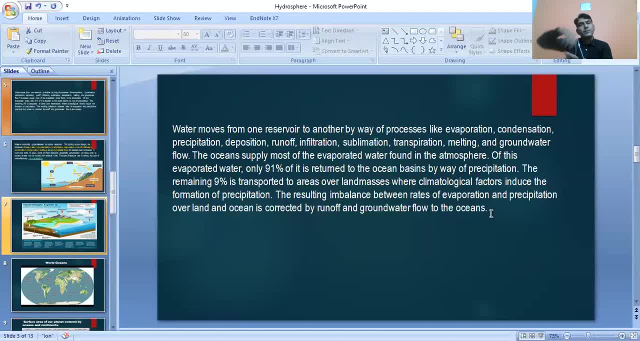 percolate, which goes inside the earth, or infiltrate, or some percent of water, some amount of water start to move or run off, so slowly in case you look- gradually under the influence of gravity, or slow it reached to the oceans and the sea. so again, this water is being added to the ocean, but by the, by the runoff. so this 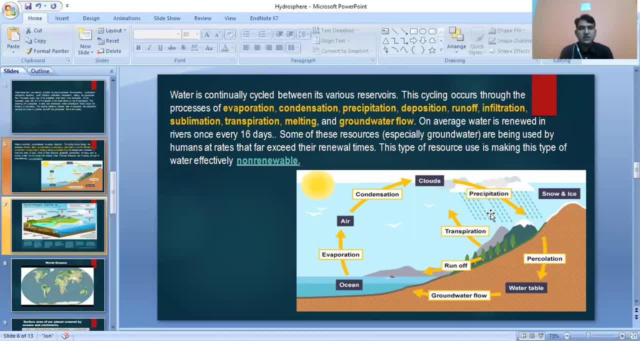 is. again, this is the conceptual framework I will I am showing in these slides. so water is continuously cycled between the ocean and the sea, but the water is constantly cycled between the in various reservoir. this cycle occurs through the process of evaporation, condensation, precipitation, deposition, runoff, infiltration, sublimation. 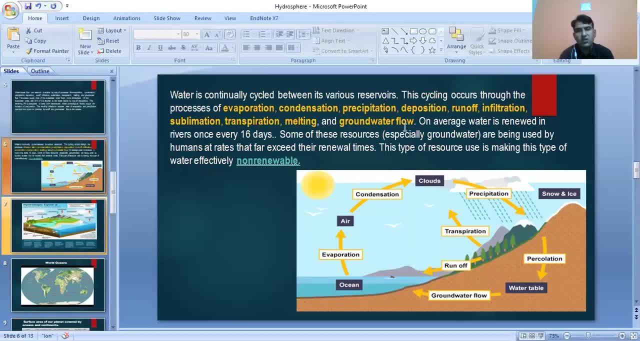 transportation, milking, transpiration, melting in the groundwater on average. so this is statement very important: on average, water is renewed rivers once every 16 days. so our rivers, by average every 16 days they get the water from through through this hydrological cycle or the water cycle. so some of these 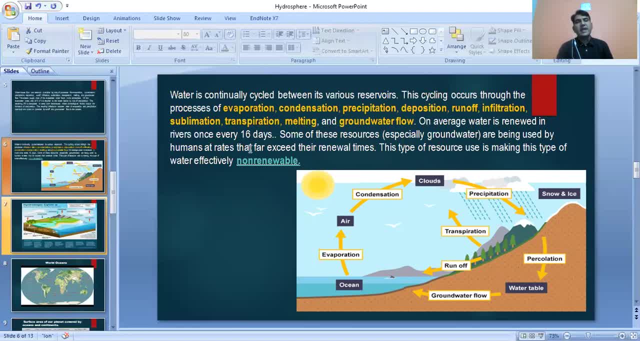 especially groundwater, are being used by human at rate that far exceed their renewable times. this type of the sources use making this type of water effectively renewable. so what this is says. look it, we have a two types of energy. one is the renewable energy, another is the non. 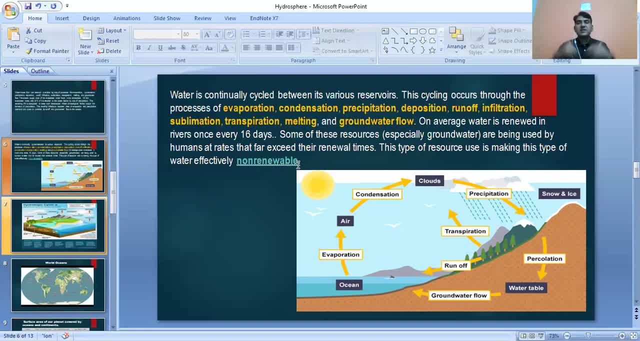 renewable energy. renewable energy is dead with regenerate which rebirth, which reoccur. so, in in this context, we have a land which is every, every time we have available land, area, land, we have all you can say soil, another soil also been part of the lane. we have a air, we have a water. so these are being considered, the 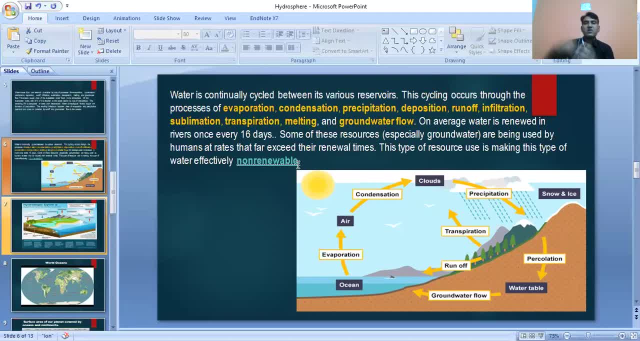 renewable energy and we have a non-renewable energy. non-renewable energies means they are in limiting amount. they are limit, they are being restricted. once we are being using them there are less chances of reoccurrence, a reproduction. so they are they once we consume them, we use them. they are not going to be regional, so it 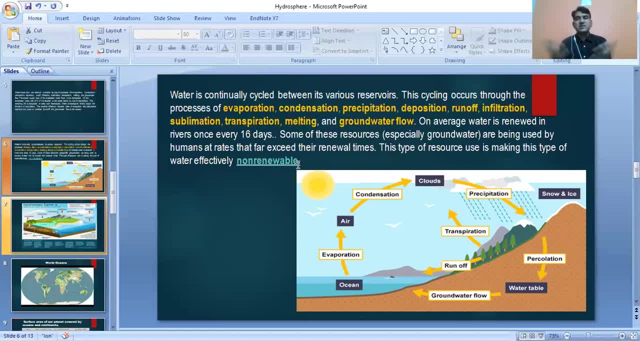 takes lots of time- of regional, so fossils, fields, one of them the minerals which are we. we are being using of them, so these are not so here. what is being saying that some? there, the water becomes a non-renewable. non-renewable because the way we are being using the water, because you, you know the population. 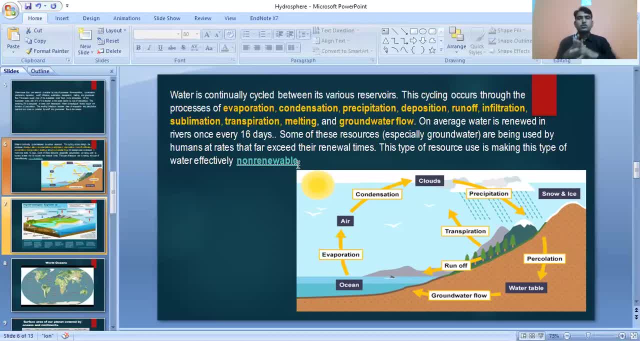 our population has been increasing, exceeding so when we compare the population and supply water everywhere we waters, however, mean so in this case, when we are being using that water in a, you know what we required and what are the supplement as a supply. something made our supply or water different. so is 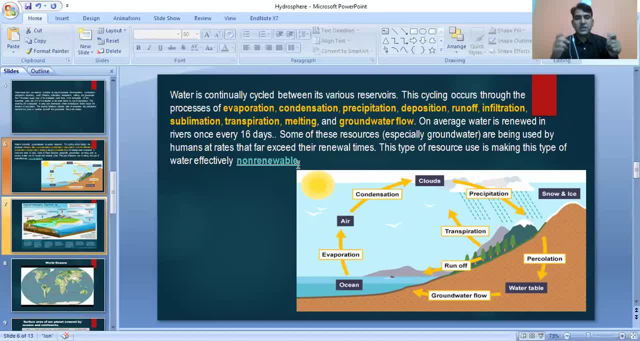 been exceeding. so in this case the water becomes the non-renewable power. so we need to have a more careful, more conscious in the consumption and the use of the water. so this is the conceptual framework of the hydrological cycle. so look at, this is the groundwater or the ocean water. so from ocean water, the 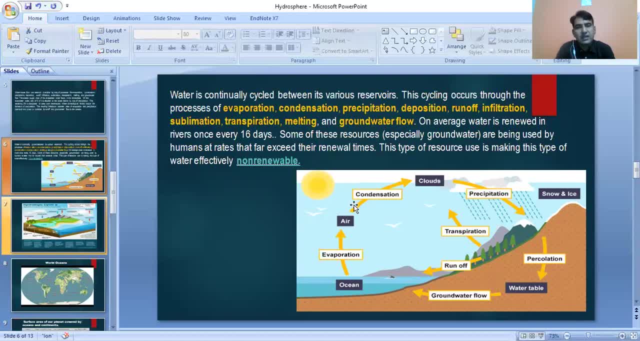 water start to evaporate, it goes into the air. then it condenses, condense there from the clouds. the clouds start to burst, then precipitation rainfall happens, so water comes down at the surface. so look at when the water is coming down, we start to run off and on slopes because, you know, oceans are. 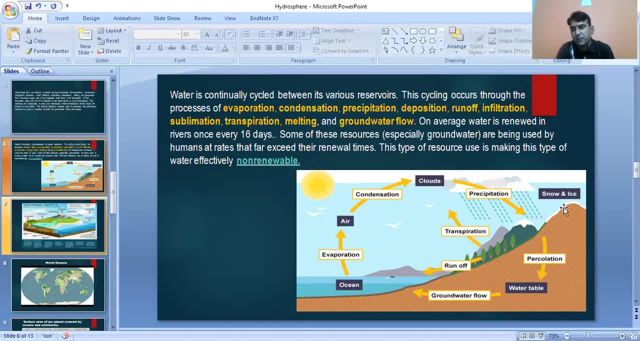 always in downwards and the landmass areas upwards. so they have always the water table of oceans, because the height has been, you know, determined with the ocean table. so landmass will always be there, so they have a height there. so under the influence of slope or the gravity, the water start to run off again, become part. 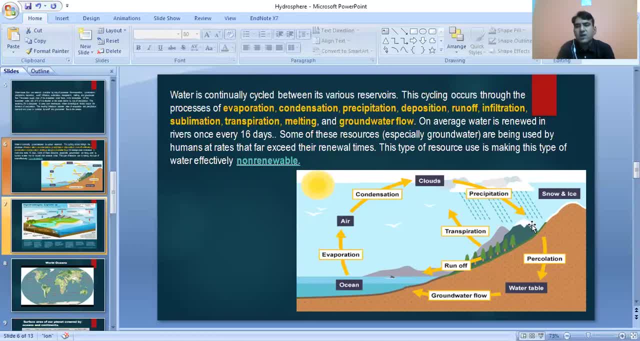 of the ocean. so some, some portion of water has been percolate. it goes inside, which is called the personal percolation or infiltration, become the what part of the groundwater, of subsurface water. some again the water has been which has been in the particip in the plants or soil. it again goes upward. it is in the form of. 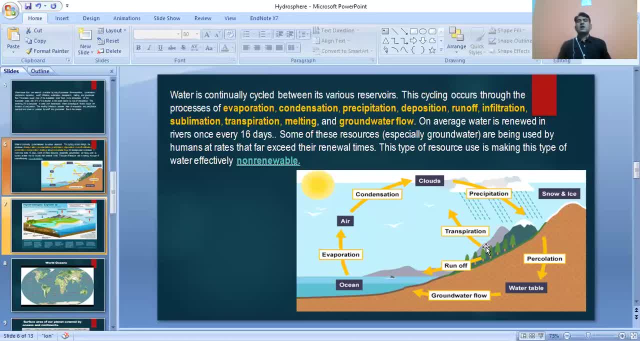 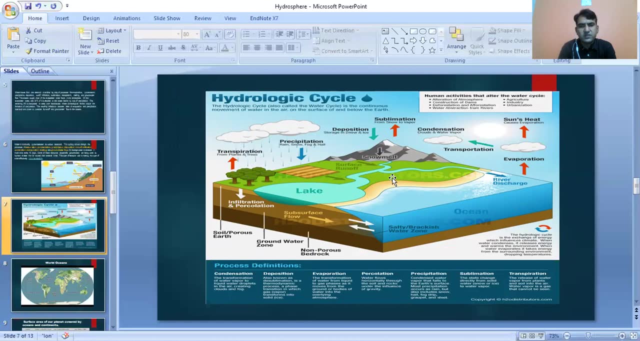 transpiration. so this process, when the water comes, comes up, are coming out from the plants. we call this process process evapotranspiration. so I hope you understand this conception. so this is the same thing you might see: transportation, precipitation, depositions. so we'll go one by one this: 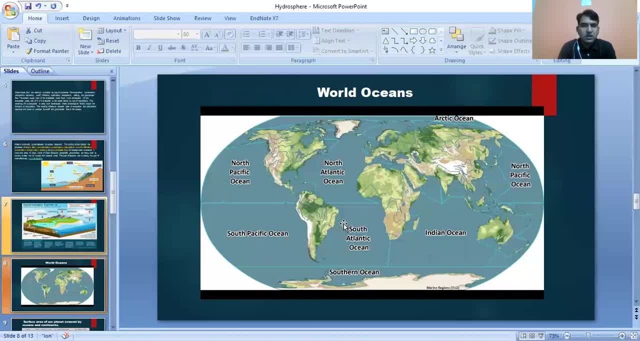 is the same thing in hydrological cycle is you know? we said that the ocean waters are important. most of the evaporation happens at the oceans, water, so oceans are the main source of evaporation. are, you can say, hydrological cycle? so even the landmass area? they get the fresh water from the oceans. so once 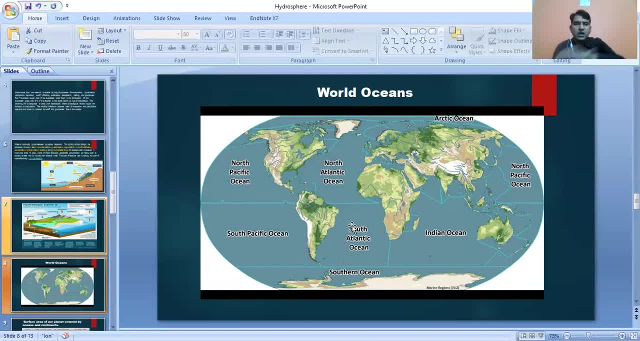 the water is being evaporated and then condensed in the precipitate. so here we just have to see the understanding, the location of these, the, what is it? these portions. so these are the world oceans, how much we have. so we have an Indian ocean, we have a south atlantic ocean, we have southern ocean, south pacific ocean, north pacific. 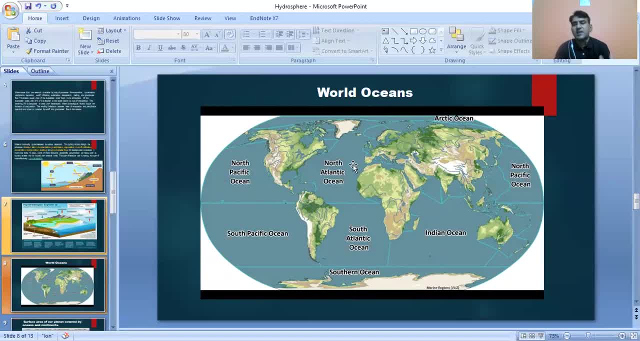 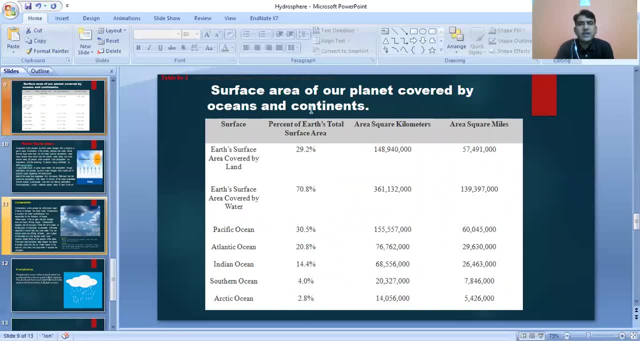 ocean we have a heart education. we'll see how much water and percentage or area they've been covering. so surface area of our planet covered by the oceans in the continent. so look at uh as surface or the land mass area or land covered, 29, the rest of the covered by the. 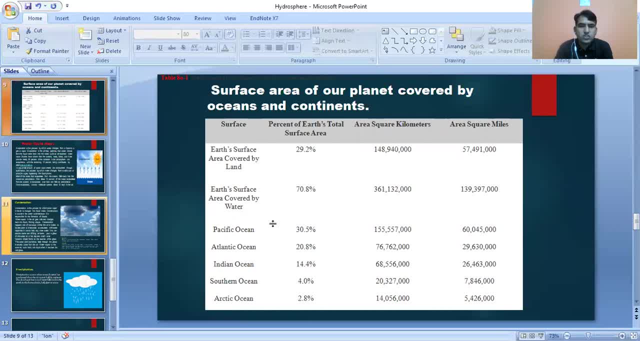 waters, water of the oceans, so this whole water. so so, pacific ocean, which is the biggest of all, uh it contains or it covered, i'll say 30 percent, almost 30 percent, more than 30 percent of uh, you know, water or the land area. then we have atlantic ocean, which is a 20, 20 percent of uh water, water. 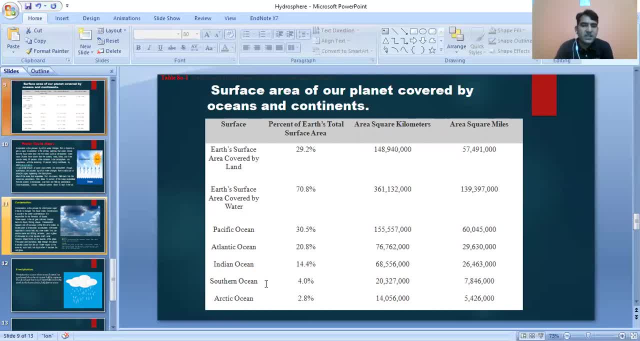 area: indian ocean, which is four, which covering 14 percent, and the southern ocean, which cuts in four percent, and the arctic ocean would contain 2.8 percent of the pacific ocean, which is four percent of the pacific number one. then we have atlantic ocean, so 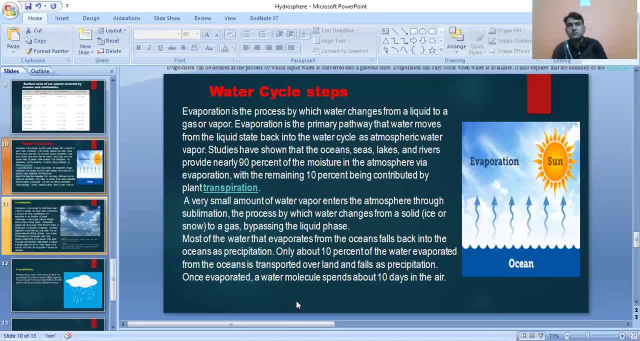 here is the first step of water cycle. uh, water cycle start from the evaporation. evaporation is the first step in the water cycle. so evaporation is the process by which water change from liquid to the gas, gaseous or in the vapor form. so, uh, you know, the water is present at the surface of earth in the form of droplets, in. 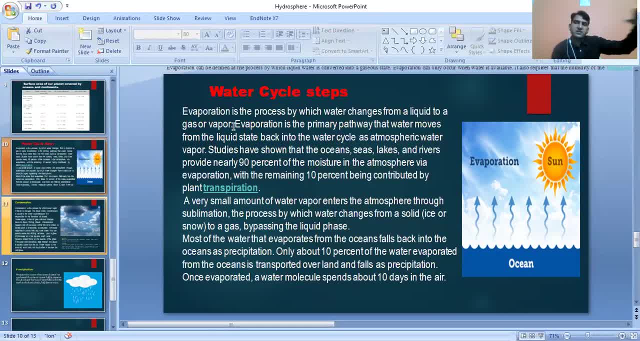 the form of water and the surface of the earth is present in the form of droplets, in the form of liquid, either in the oceans or in the river, seas, ponds, even the, even the soil, water, so that water start to evaporate, it changes state, from uh, from liquid to the case or the vapor, and they start to 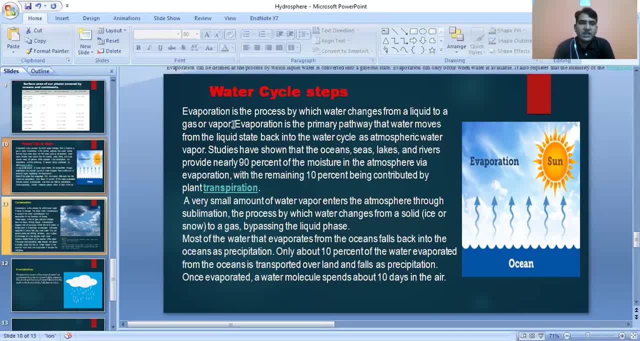 move further up in the in the environment or in the atmosphere. so evaporation is the primary pathway that water moves from the liquid state back into the water cycle is atmospheric water. studies have shown that the ocean, seas, lakes, rivers provide the most water for the environment- nearly 90 percent of moisture in the atmosphere- via evaporation, with the remaining 10 percent 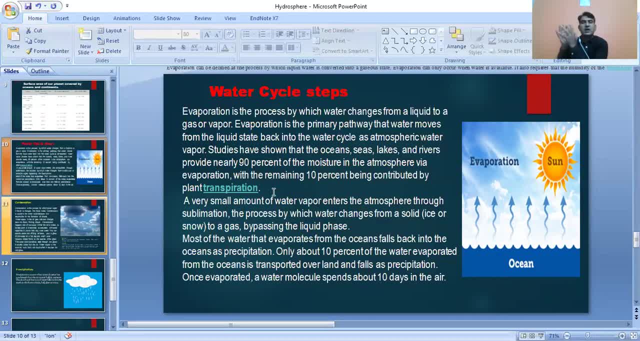 being contributed by the plant transpiration. so about 90 percent of water, transport water has been evaporated from the, from the ocean and uh, from the ocean, seas, lakes, and the rest of 10 percent comes from the plants, which process called the transpiration. so that you know the plants, uh the. 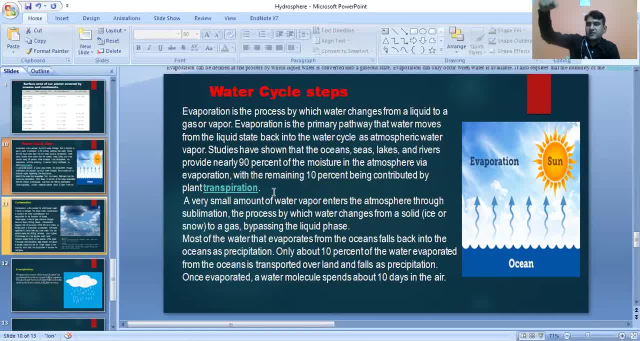 what you say. the leaves of the plants are porous one, whichever, whichever, whichever openings, from these openings, the water is being coming out in the form, which is which processes are called the transpiration. when the sunlight is being on, and you know the, the roots are always being downward and down. 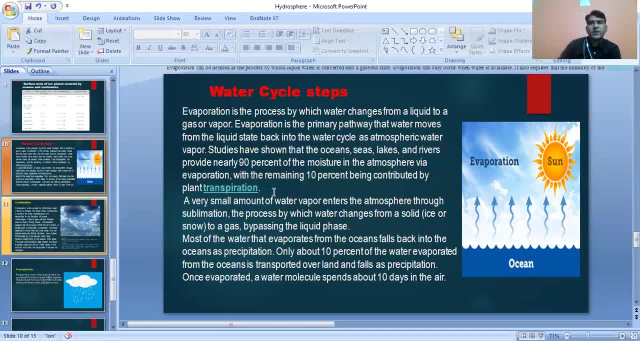 beneath the earth. uh, some, some plants are deep rotates, some are modern rotates, so roots are always being at the bottom. so through this the water has been, you know, uh goes upward in the, in the sky, in the form of transpiration. a very small amount, a very small amount of water vapor enter the atmosphere. 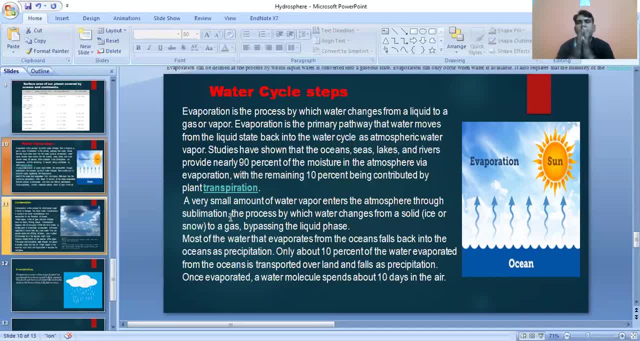 through the sublimation. as i told you, sublimation is a process by which water convert directly from from solid to the vapor form. so most of the you know, top of the peaks of top or peaks of the mountains where there is a ice, ice has been there. so those that ice, you know that ice convert. 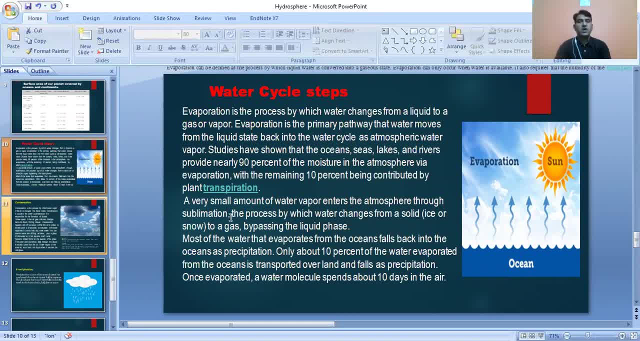 into the vapors and directly goes in the environment of the atmosphere. so the process by which water changes from a solid ice outer case bypass in the look at first. so the third, the second phase: when we have our eyes, they convert on the look at and look at. 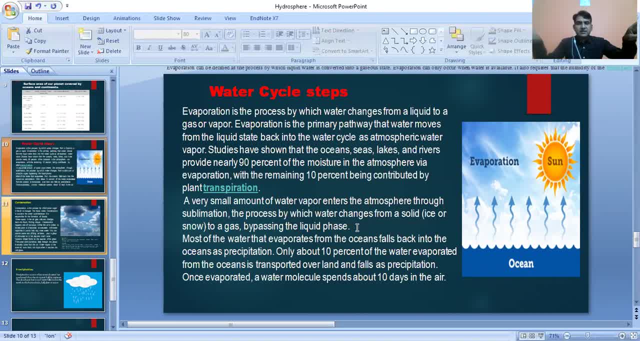 convert to the cases. so it in the, the sublimation process, leaves, uh, leaves. the second process of solidification means where the solid is happening, means look at form. so look at form is being gone so. so in this case it directly converting from solid to the gas. so there's no look at phase. so 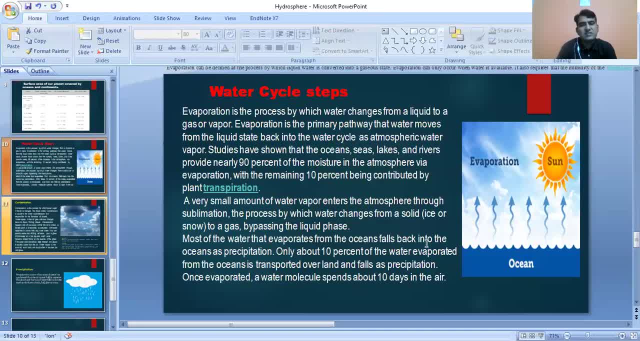 here. so most of water then evaporate from the ocean falls back into the oceans is a precipitation, fine. only 10 percent of water evaporate from the oceans is transported over the land, falls in precipitation. i told you. 90 percent fall in the on the oceans and 10 percent goes to the landmass. 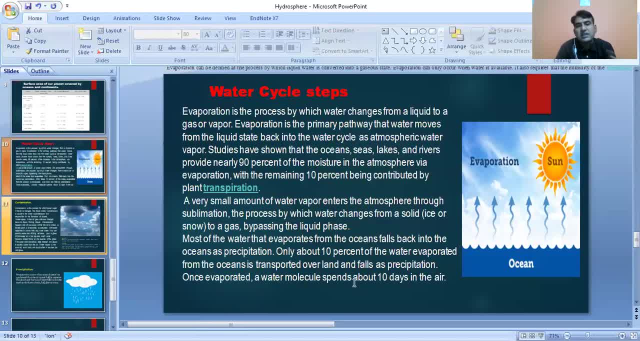 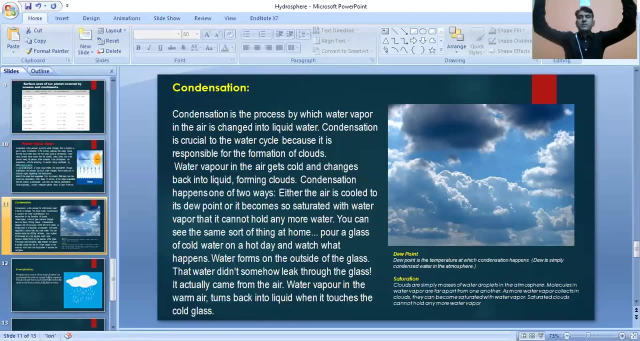 area. so once evaporated water molecules spans about 10 days in the air. so when the water evaporates they can remain in the environment for the 10 days. so this is the. so again, that was the first process. when the water goes up in the form of vapor and 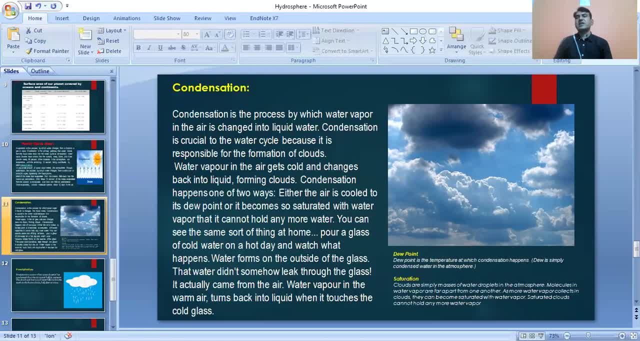 and is always being available in the environment or in the indian atmosphere. so what happened? the next step is the condensation is the end of the process. so condensation is the process by which water vapor in the air is changed into the liquid, so dead water, which was in the vapor. 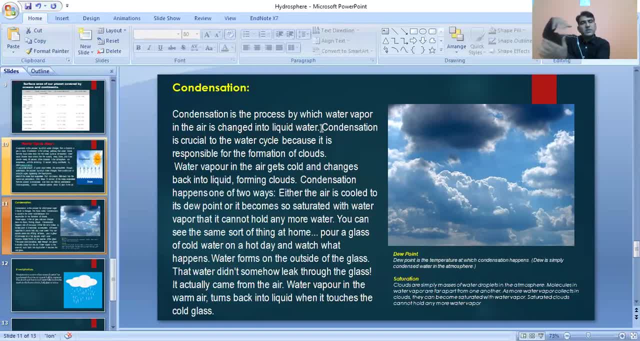 form again has been changing in the liquid form. so once it's been changing from vapor to the liquid, then refrigeration, which is in the water form, so its condensation is inside, means when you evaporating there is a technique of meaningful growth for body from water. so it's called the 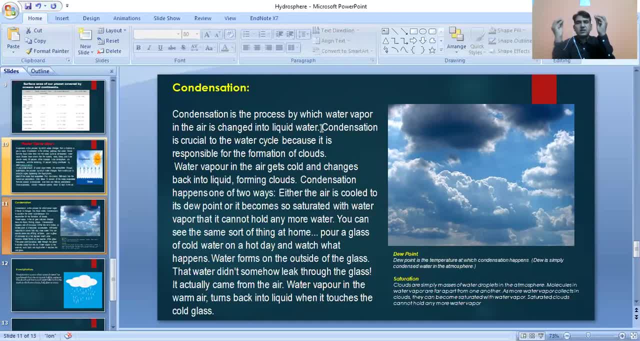 condensation process. so condensation process is based on the clouds, where the clouds are being formed so that water evaporates under certain conditions. the quasi call circuit together, our closed together. we will see this process. so water vapor in the air gets cold or change, baking into. 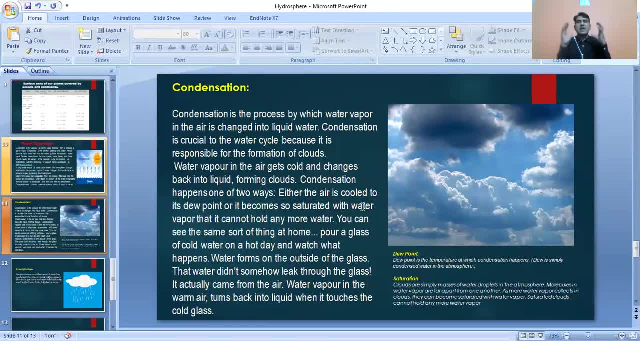 the liquid forming the gloves. condensation happens one other two ways: either in the air, is cool to due in stupor, or becomes social. so the condensation happens because of the condensation process. we see two ways. It is a two factor or the two ways. One is the dew point and there's a 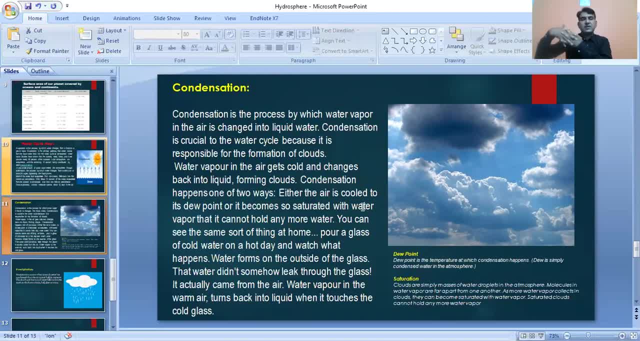 saturation point. Either the you know the air is being reached to the dew point. Dew point is the condition of the temperature, means there's a low temperature, or you can say cold temperature, where that vapor start to convert into the liquid. Another state is saturation. Saturation, the condition of. 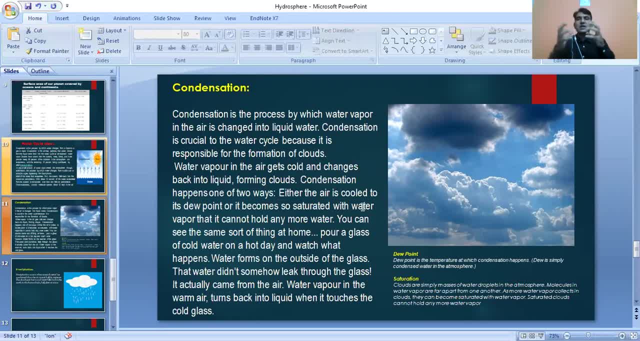 the air, where water- sorry, where the air could not held more water. So what happens when these, when the vapours goes up, when they start to combine together, start to close together and they make the droplets So in the clouds. so those cloud doesn't have a more capacity because there they. 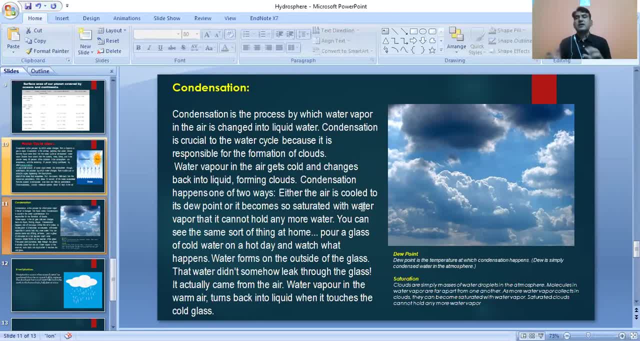 are already saturated. So once, once that the other droplets will be will be part of the condensation, part of those clouds. the clouds start to burst. So what is that Means? cloud clouds don't have a capacity to hold more, more water. 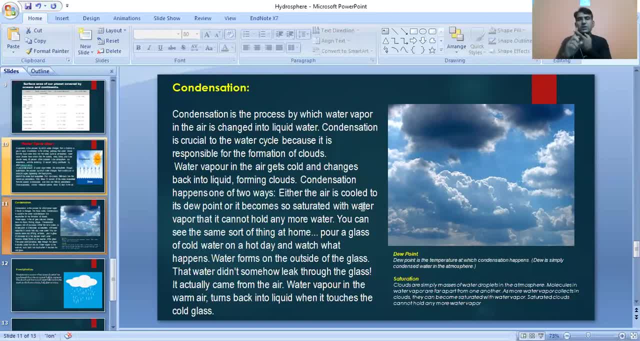 So this is called the saturation. So the condensation happen because happens of the two ways, because of two ways. One is the dew point. Dew points relate to the temperature and the saturation. saturation relate to the saturation means the holding capacity of the air. 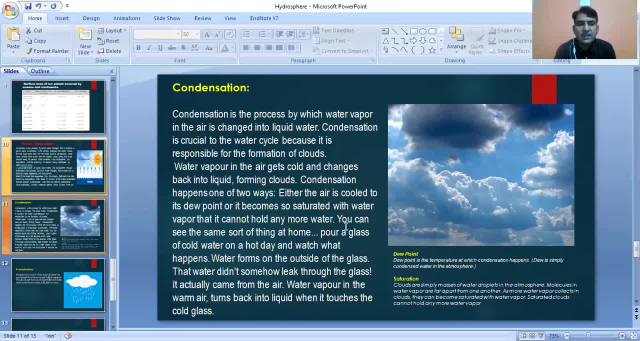 So one is the temperature and another is the air. It is similar, like you know, if the example is given here, that when you, when you have a cold glass of water, when you pour the, what is it? the cold water in the glass, and 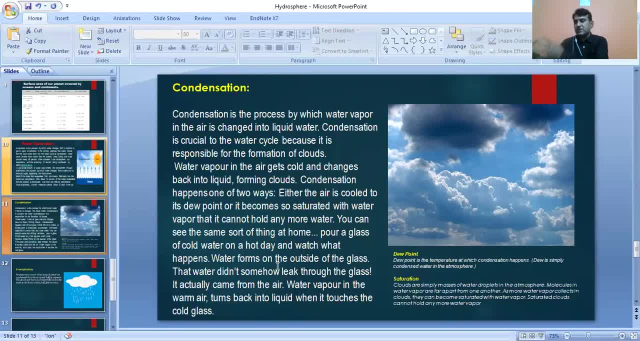 you put that water, that glass in an area which is warmer one, So what will happen is the outside corner of the glass, they will have a droplet. So what happens? The the outer, the outer environment, Because you know, in the, in the environment, on the air, it is always vapor. 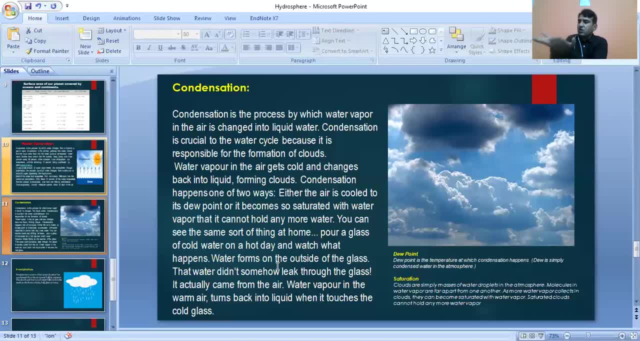 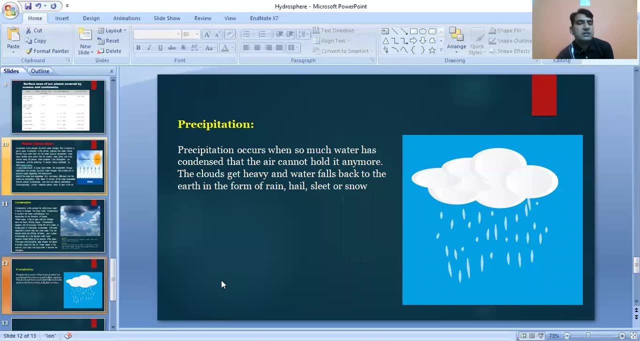 So when the vapor, they would find the lower temperature, because low temperature is it at the corners, at the corner, at the sides of the glass. So then by the case they convert those vapor into the droplet. So similar happens here in the condensation process. 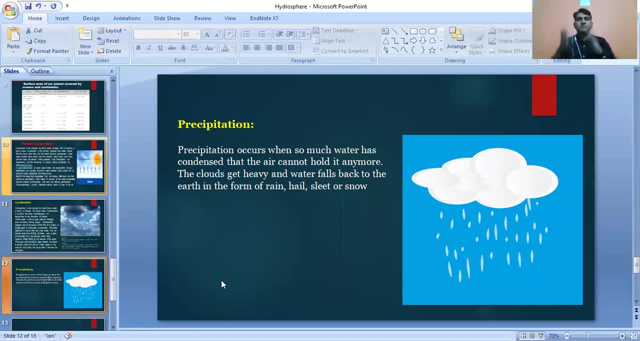 Number third is the precipitation. So we had an evaporation, condensation, now the precipitation. What is precipitation? What is precipitation? Precipitation occurs when so much water has condensed, when the water has been contained, there are lots of clouds, they, they, the, they have made or formed the clouds and those. 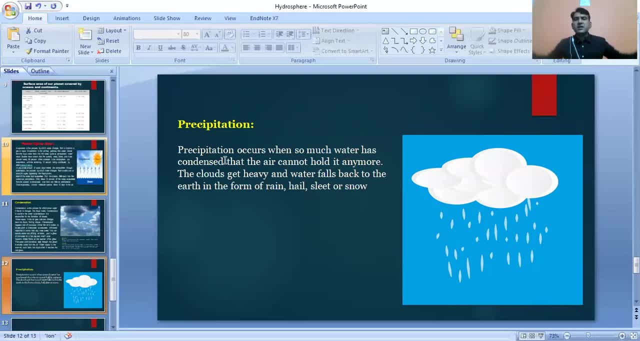 clouds are. those clouds are almost saturated and reach on the dew points and the air cannot hold anymore. So in this case, whatever, the clouds get heavy and water falls back into the atmosphere. So when these clouds start to burst, they give water. 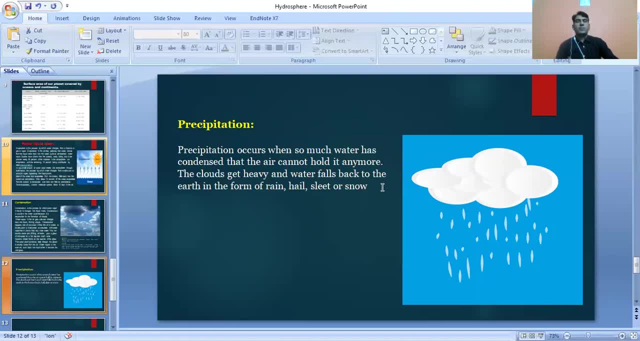 That process is called the precipitation. Precipitation means the uh, in other words, they are being called the rainfall. But that precipitation comes in different forms. One is the rain, Another is the hail, Hail, uh, you can see the. what do you say? something like the uh, bigger, uh, jo jo. 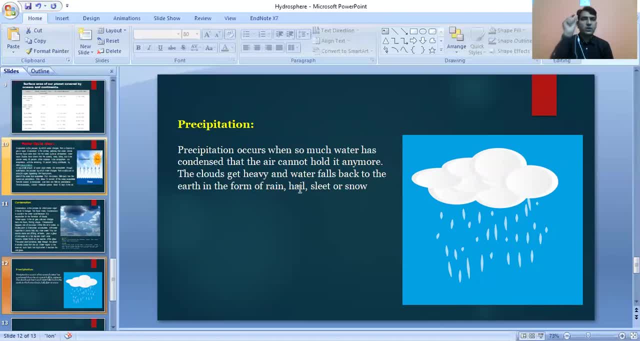 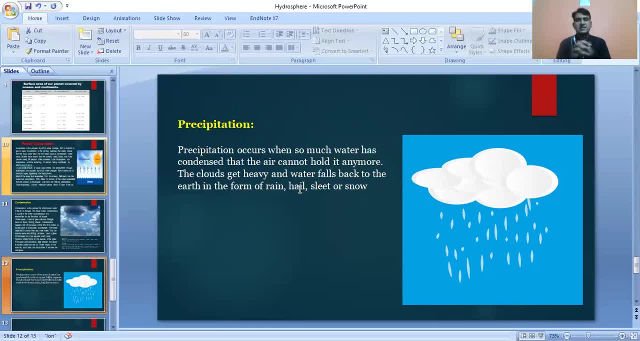 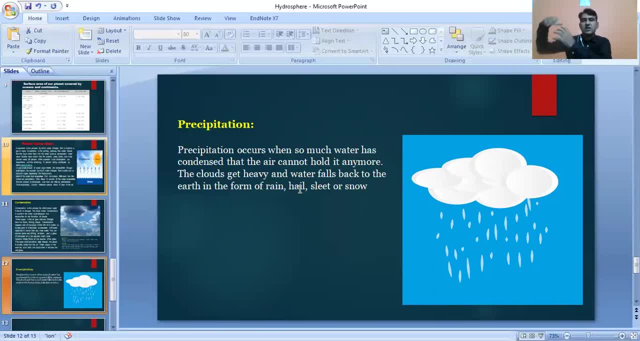 So we have a mixture of both uh snow and the drops, So we call it the sleet. sometime, you, you, you, experiencing the uh uh, the rainfall, the same time we have a single fall Dead slitting is not like a hail or the snow. 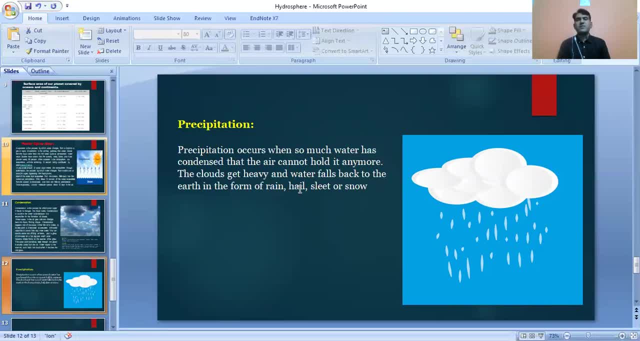 It is similar, like a very puffy type of snow falling and with the rainwater. And number 10 is a synov Directly synov is coming from, So when the droplets are coming from the top, from the atmosphere, they find the low temperature. 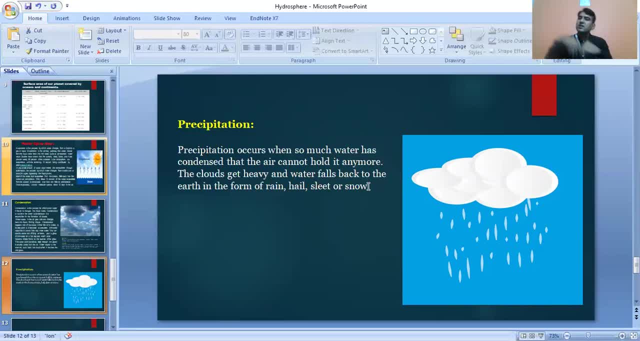 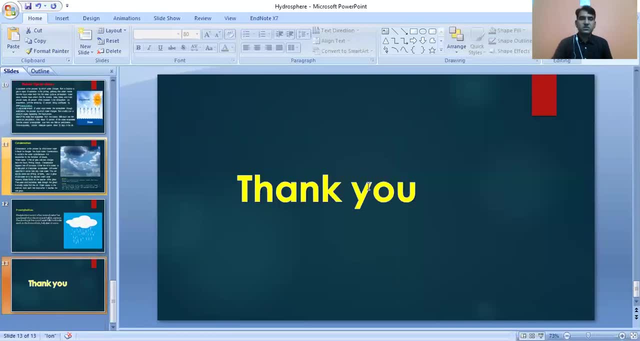 They are coming from the top and they find the low temperature on the way. They convert from liquid to the solid form and they convert in the synov and they fall on the ground. So thank you very much. It was all about the hydrological cycle or the water cycle. 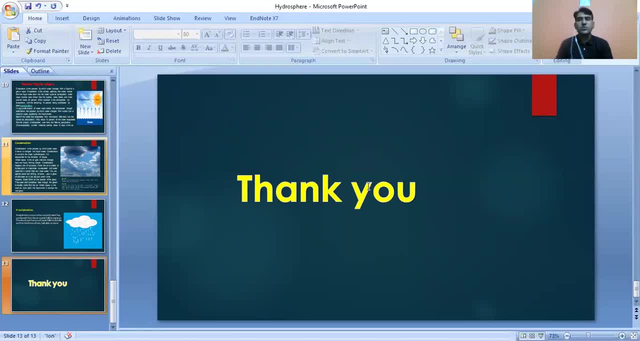 which was important for us to discuss here. I hope you understood that. So we will come out with another video in the future. So till then, thank you very much and take care of yourself. I hope you understand. This is all, Thank you.